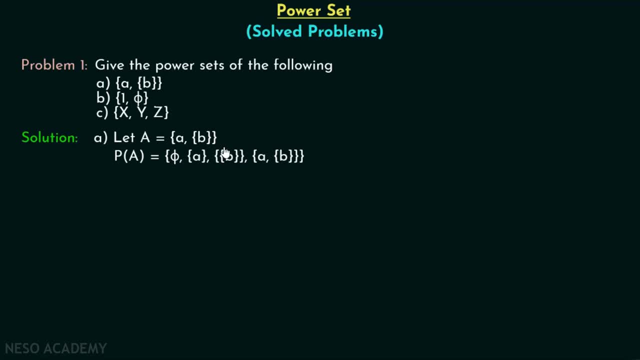 And this is another set with this element, that is, a set with element B Right. Obviously, this is an element of this set A. We have to form a set with this whole set Right. After this, we can create a set with two elements. these two included. 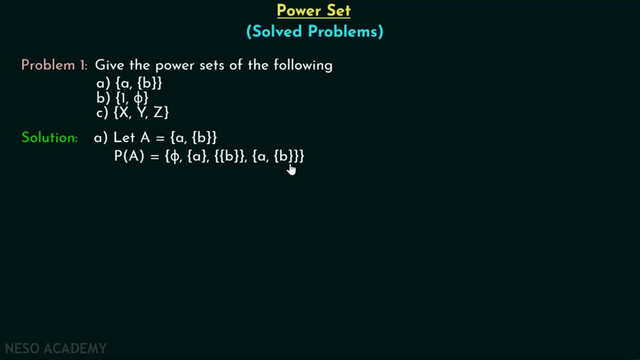 As you can see over here, this is how it looks like, Right? So it is clear that this is power set of A, which consists of all subsets of this set. Right Now, here you can see, this is a set with two elements, one and phi. 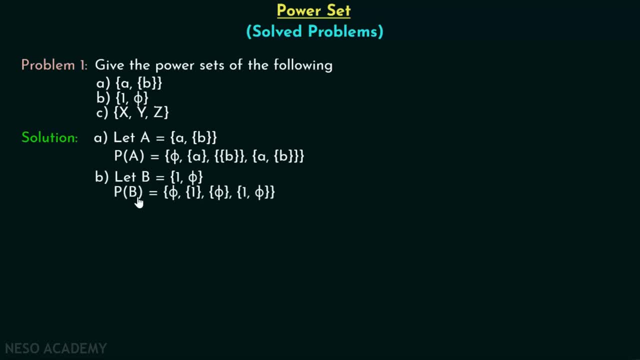 Let B denotes one comma, phi. that is this set. Okay, Power set of B must include phi, which must always be included Right After this. we can form sets with one element. You can see I have formed these sets with one element. 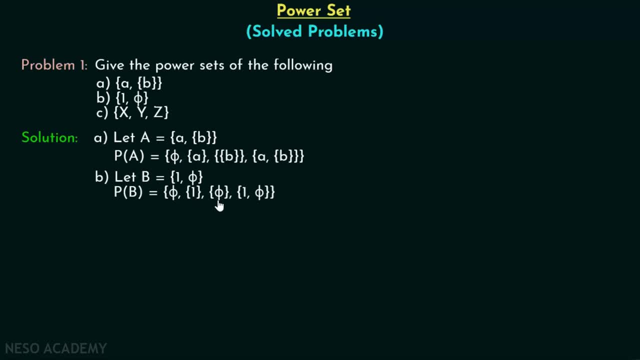 One is one, the other one is phi. Right After this we can form a set with two elements, that is one, comma, phi, as you can see over here, Right. So this is power set of B. Now let us suppose that this set is represented by C, capital C. 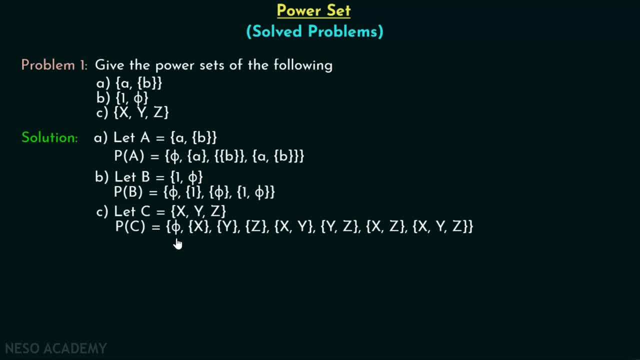 Then the power set of the C must include phi. After this sets with just one element, as you can see, X Y Z. Then sets with two elements: X comma Y, Y comma Z, X comma Z. These are the possible combinations. 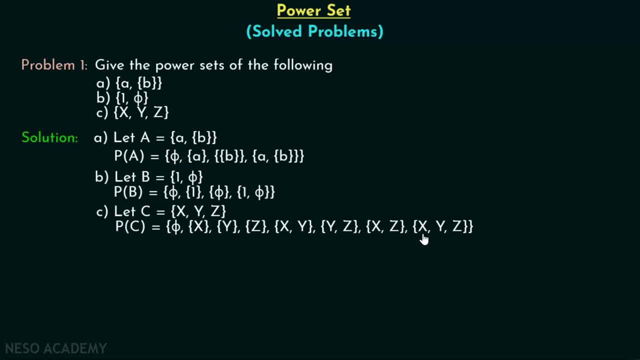 Right, You should include every possible combination After this: a set with three elements. Right, This is power set of C And obviously you can see there are total eight elements in this set. Always check the number of elements in the set. 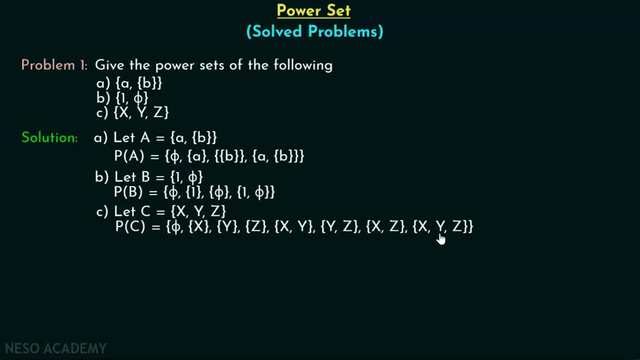 Okay, If there are three elements here, then there must be eight elements in the power set of this set. Fine, If there are two elements, then there must be four elements in the power set of that set. Okay, Now let us discuss problem two. 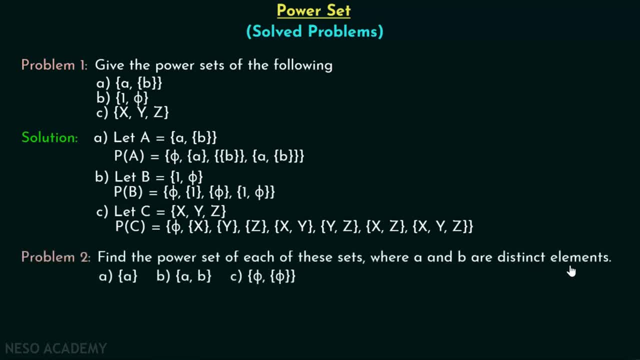 Find the power set of each of these sets where A and B are distinct elements. Okay, So we have to find the power set of each of these sets. Let us suppose that A represents this set, Then obviously the power set of A must include phi as well as this whole set. 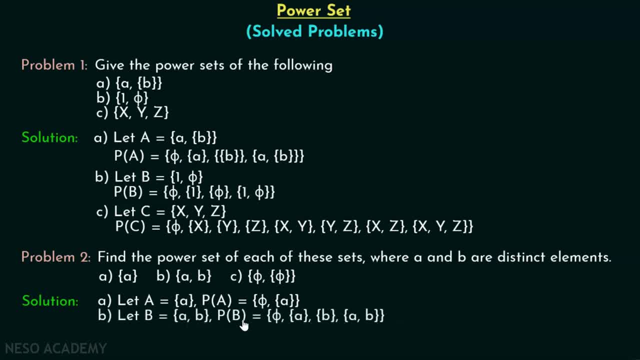 Let us suppose that B represents this particular set, Then power set of B must include phi sets with one element and obviously a set with two elements. Right, This is power set of this set. And let us suppose that C represents this set. 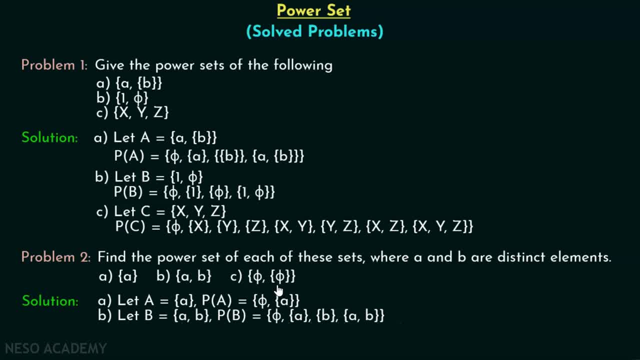 And you can see there are two elements in this set. So obviously power set of this set must include four elements. Here these two elements are phi and a set with phi Right. So obviously the first element of power set of C must include phi, which is obviously included. 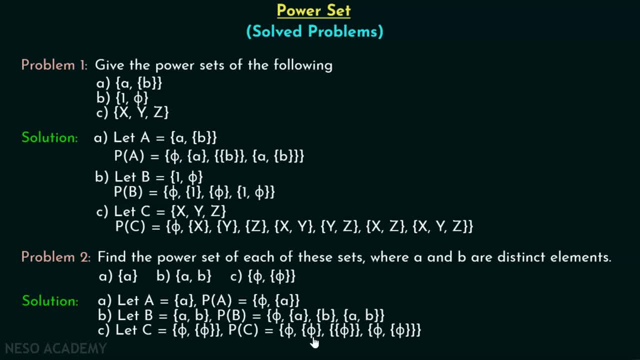 Then we will form sets with one element. The first element is phi, So we will include this phi within a set. Second element is a set with phi Right, So we will include this set with phi inside another set. And then we can form a set with two elements, that is, phi and a set with phi. 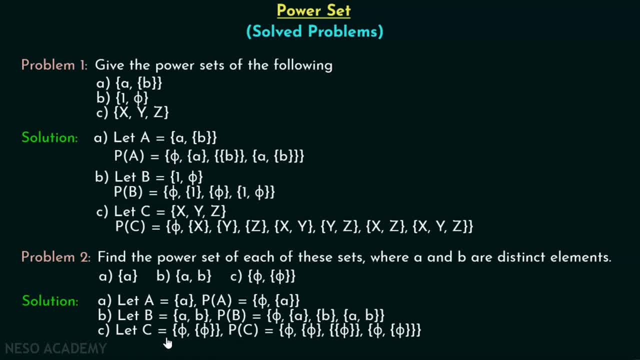 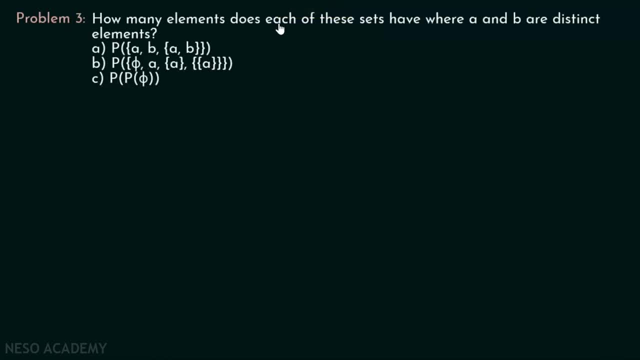 Right, As you can see over here, This is power set of set C. Fine, I hope it is easier for you now. Right Now, let us discuss one more problem. Here is problem three: How many elements does each of these sets have, where A and B are distinct elements? 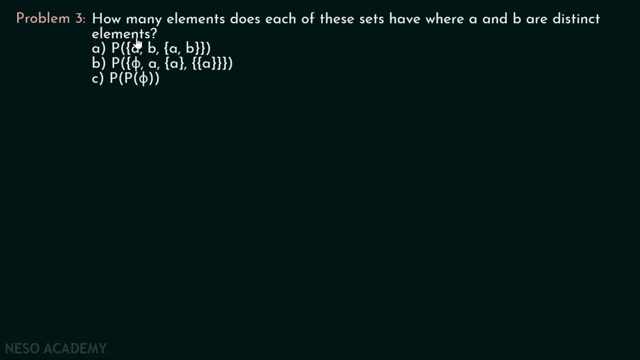 Okay, A and B are distinct elements. We have to identify how many elements does each of these sets have. Let us first discuss this. You can see it is written over here: power set of this whole set. First, we have to identify how many elements are there in this set. 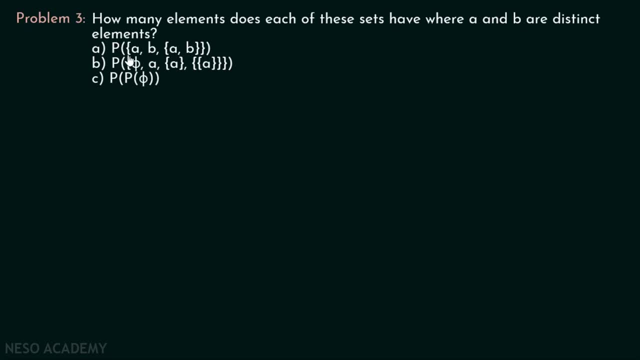 Then only we would be able to identify how many elements are there in the power set of this set. We know that this set has three elements. Right Power set of this set contains all possible subsets of this set. Therefore, power set of this set has two to the power three, that is, eight elements. 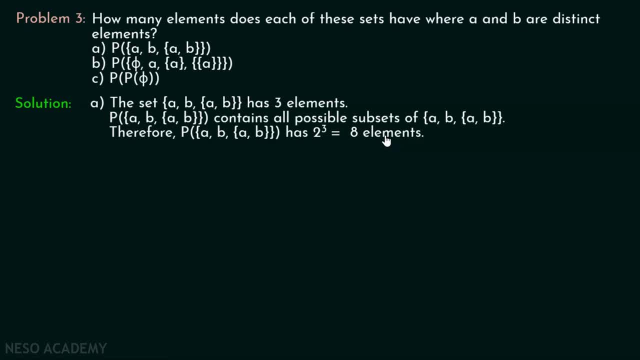 Right. So there is no doubt about this, that there must be two to the power, three, eight elements within this power set. There is no need to write them all, because in this question it has been asked that how many elements does each of these sets have? 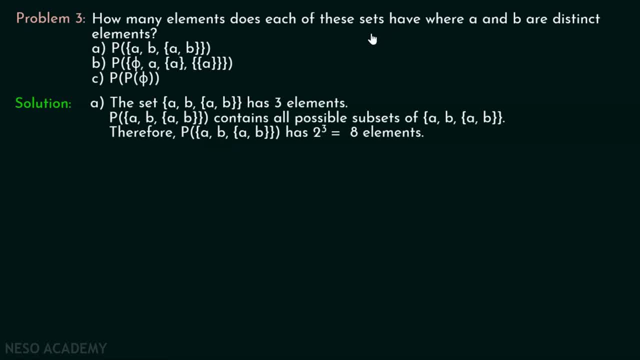 Only we have to answer how many elements are there in these power sets. Okay, Here you can see: we have a set with five A set consisting of an element A, and then we have a set with another set, and this set is holding A. So there are total four elements in this set. 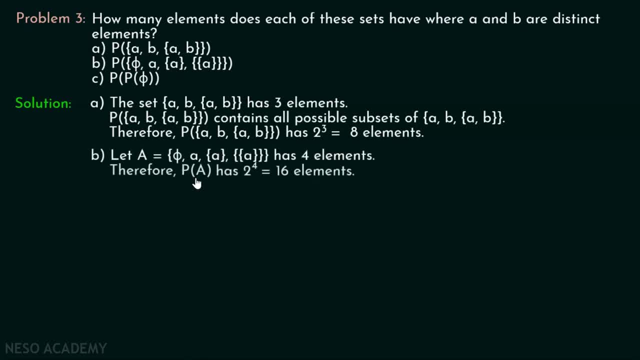 Right, Total four elements. Therefore, the power set of this set must hold sixteen elements in total. Right Now let's discuss this option. Here we are talking about power set, of power set of five. First of all, we must have to identify how many elements are there in five.